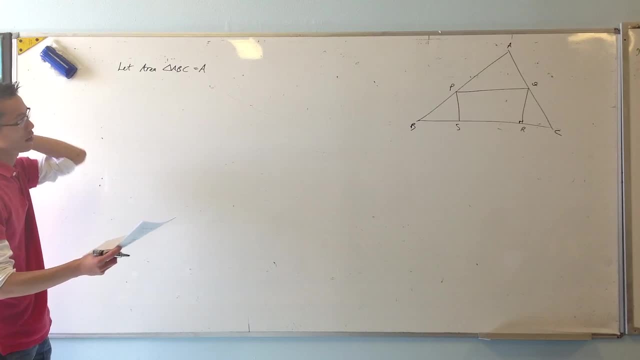 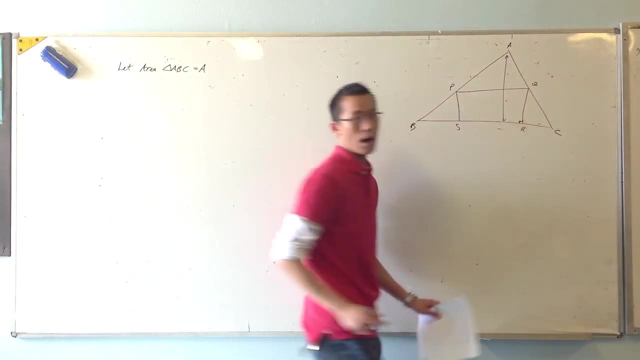 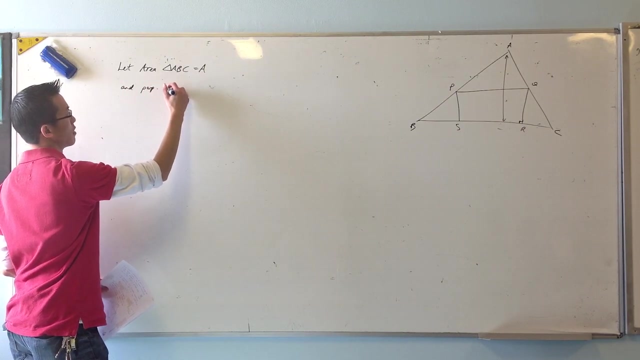 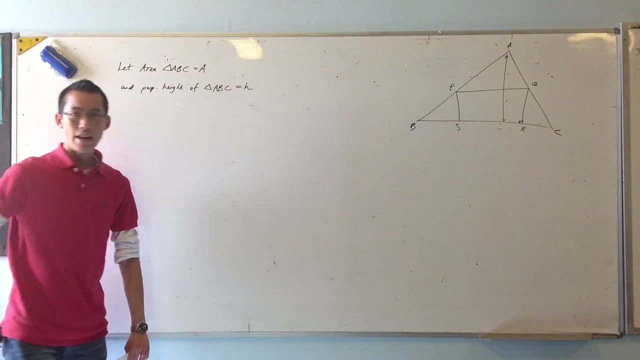 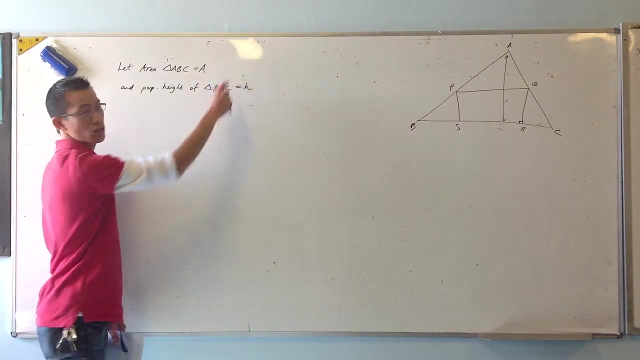 I also need to know the perpendicular height of this whole triangle. okay, so I've got this length here. I'm going to call that perpendicular height H. Now I could work out this. I could work out the base, right. but I don't need to work out the base as another variable, because the base is going to be a function of these two, right, as you'll see shortly. 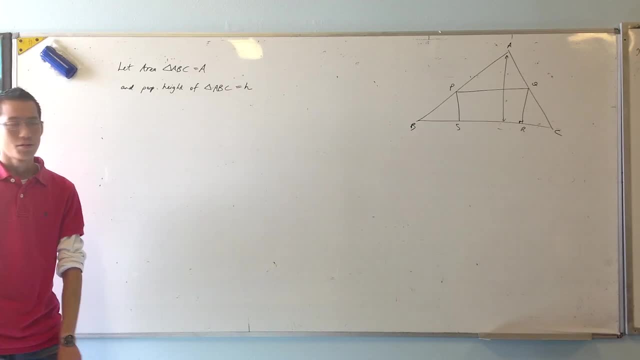 So I'm not going to introduce another variable for that Now, sorry, another constant. I really should make this capital H. Sorry, can I see great white? Yes, it's right here. Okay so capital H, constant constant. 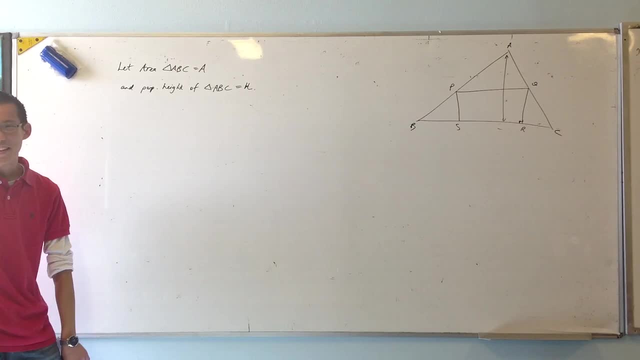 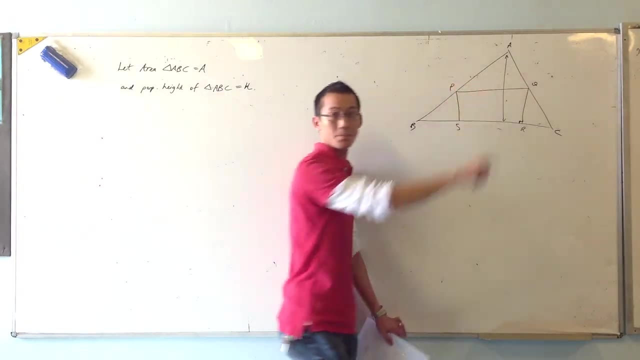 Okay, smooth. All right, let's keep going. All right, now I'll introduce the variable, I'll introduce the variable parts now. okay, Now the variable parts are the dimensions of this rectangle. okay, because they can move about and we can change it. 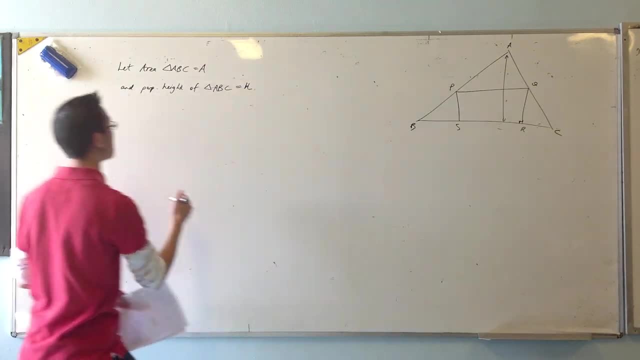 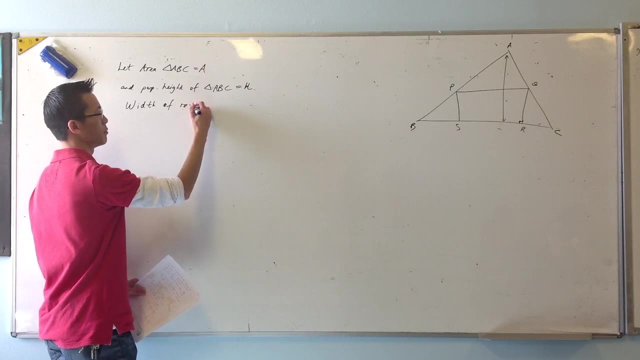 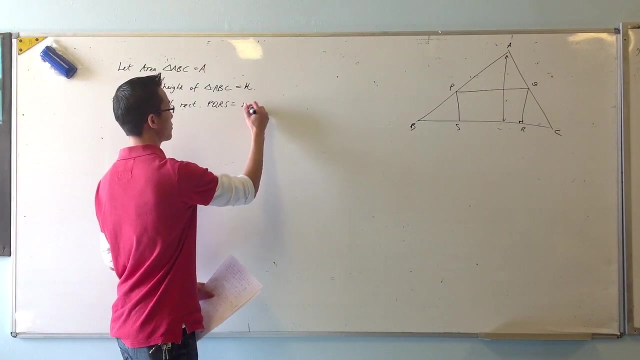 It can be a really flat one or a really tall one, that kind of thing. So I'm calling the width of the rectangle PQRS- I think I called it X, X because it's a horizontal thing, right- And the height. 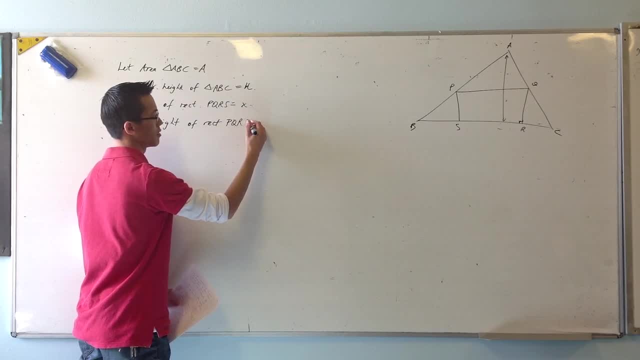 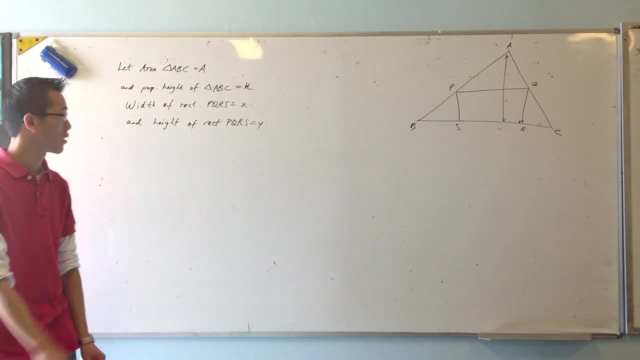 So I'm calling the width of the rectangle PQRS of the same rectangle as Y. Now the thing about these two variables is I will actually be able to get rid of one eventually, okay, but it'll take some time to get there. 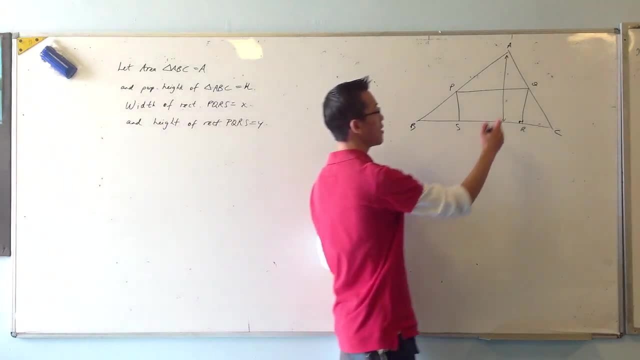 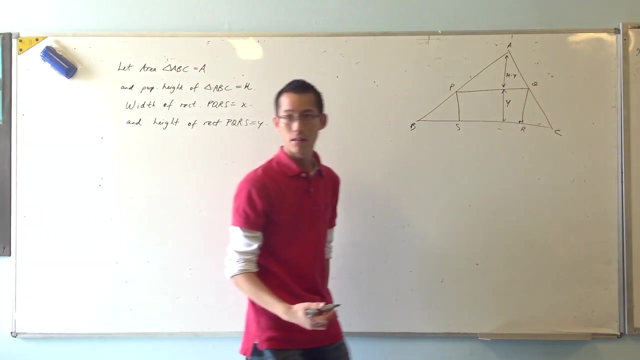 I'm going to get one in terms of the other, I'm just going to leave them there for now. So if that makes I'm going to get rid of this and this, that makes that Y right that part there. So therefore, this section up here for that little small triangle up top, will be the total height, minus that. okay. 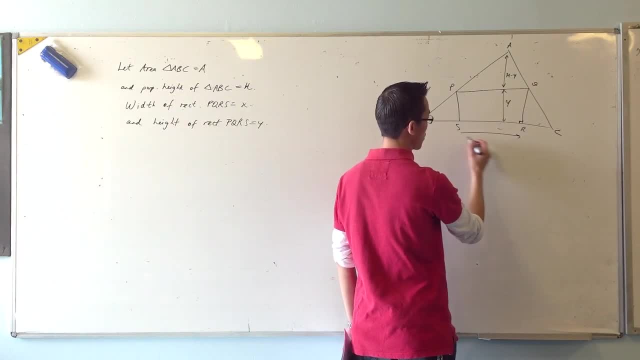 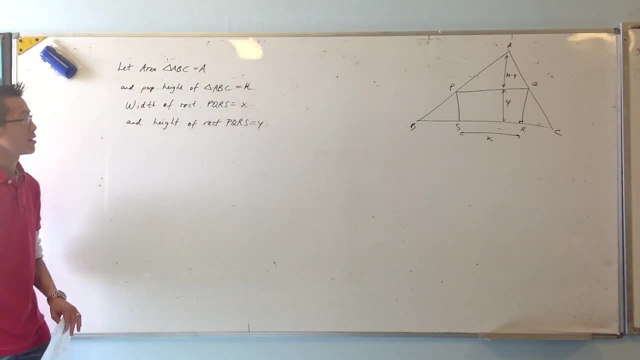 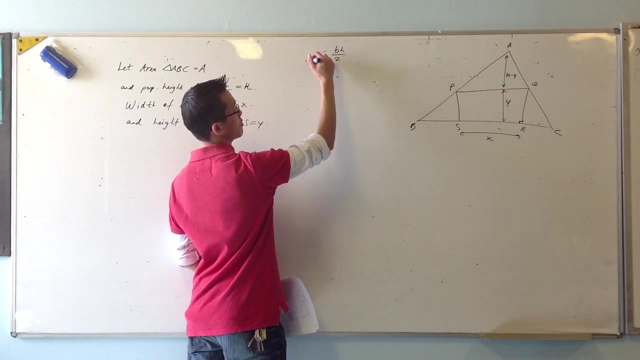 Are you happy with that so far? Now, this part across the bottom, that's going to be X, And if I want to work out that base length BC, okay, because I know the area of a triangle. right, The area of a triangle is base times, height on 2, right. 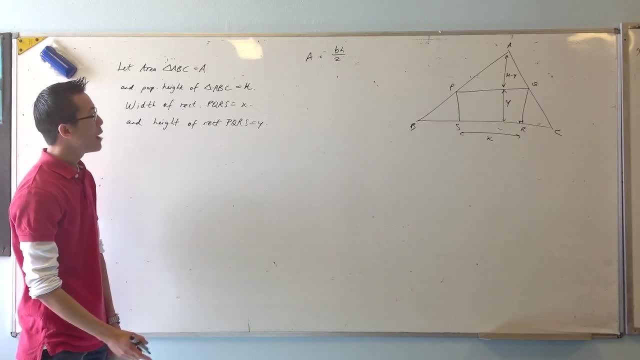 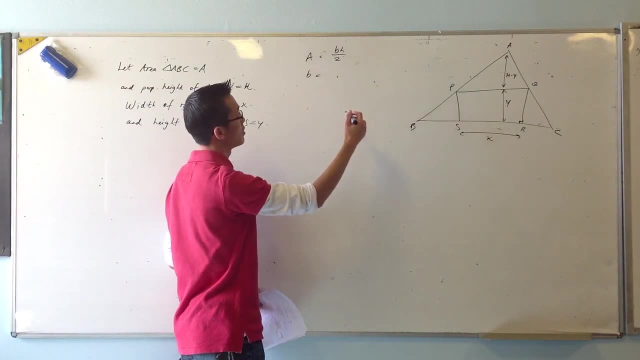 Well, my area is actually called A right. My base is what I want to work out. My height is capital H, So when I rearrange this right, the base I'm after is A Okay, 2A on H. 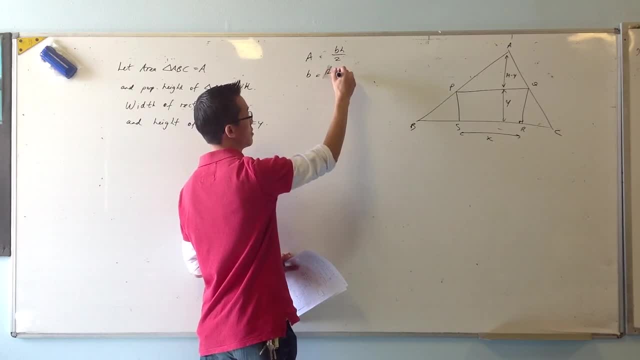 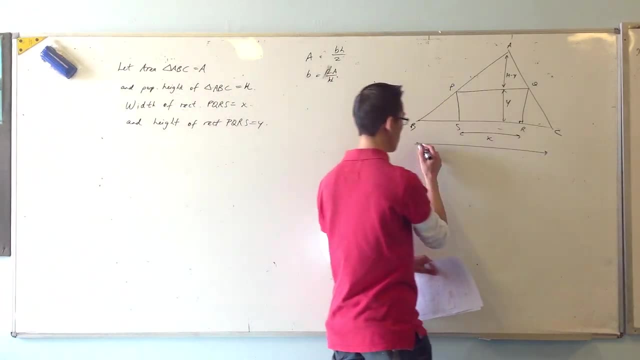 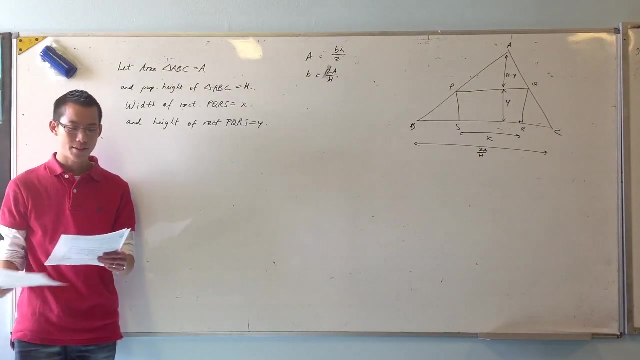 Wait, hold on. 2A on H: Yeah, 2A on H- Capital. Okay, So I'm going to call this whole way down the bottom. 2A on H: Okay, So, now I'm set up. Now, this is where the weird bit comes in. 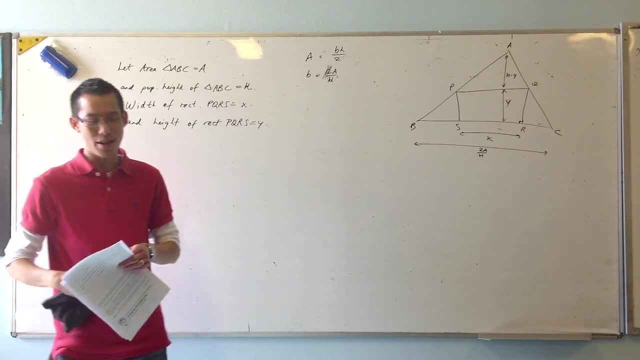 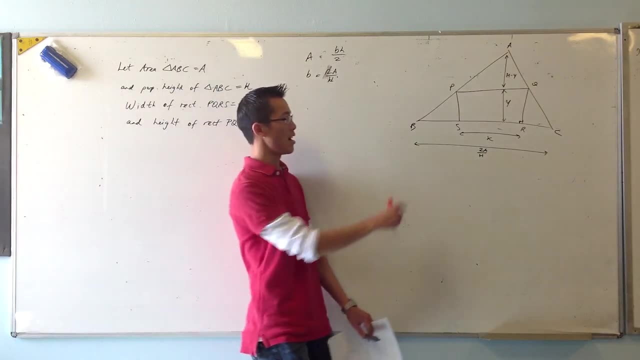 And I know some people will not be very comfortable with me doing this, but deal with it, I'm going to do it anyway. It makes things a lot easier to work with. Is that what you've got down here? this weird trapezium-looking shape here? okay, 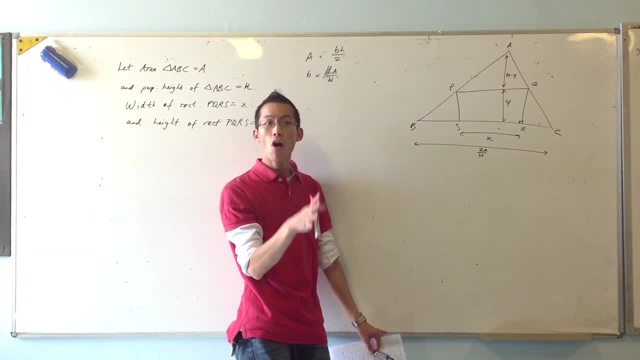 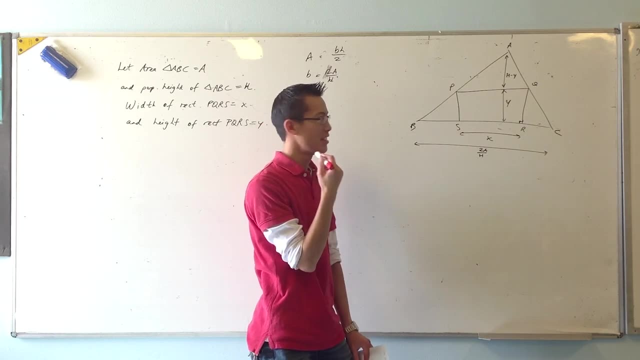 PQCB: It's trapezium, right? What I'm going to do is take that trapezium and I'm going to slice out the rectangle in the middle. Okay, You're like huh, You'll see why in a second. 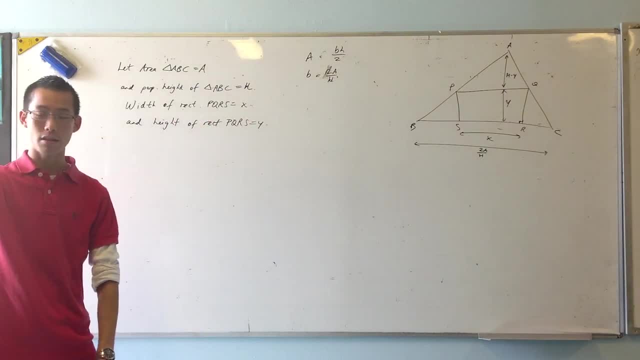 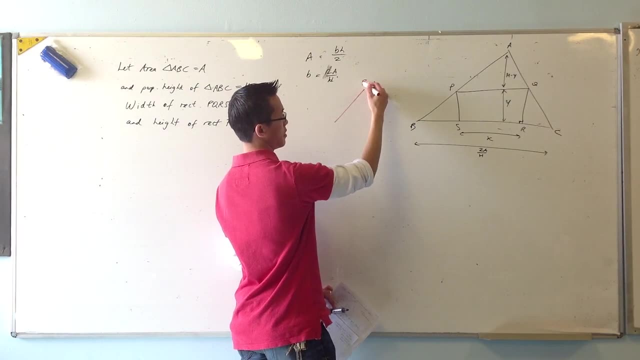 But if I take that out- which I can totally do because the rectangle right, the sides are equal- okay, What I'm going to get is this new shape P and B. Okay, This is also going to be the point Q. It's going to move over because it sort of collapses. 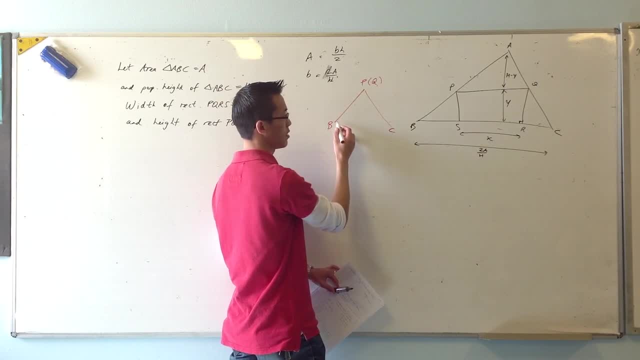 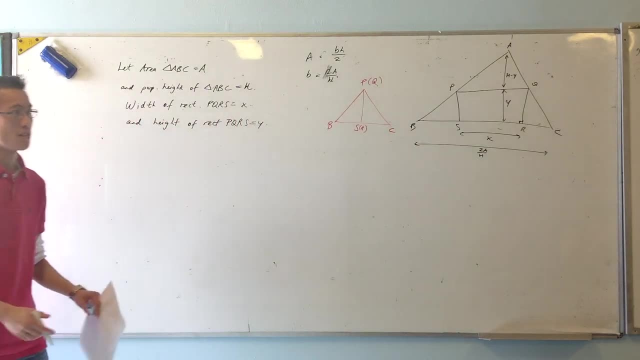 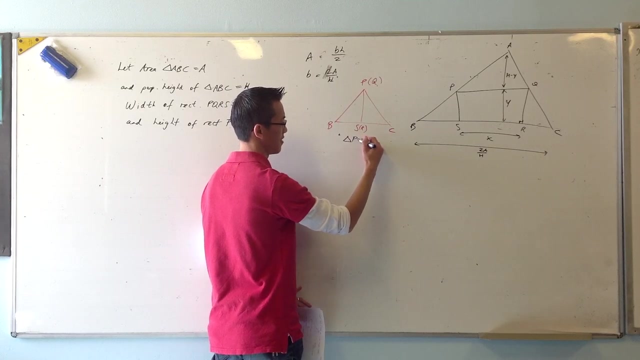 Okay, This is going to be C over here, And in the middle you've got point S. It's also point R. They're the same point. Okay, See the top of each other. Okay, So I'm going to call this triangle graceful and elegant. as usual, Grant, I'm going to 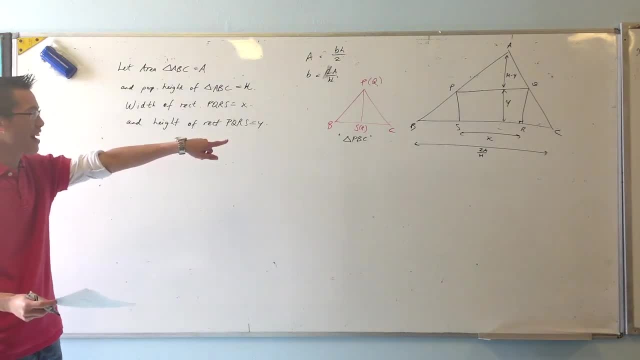 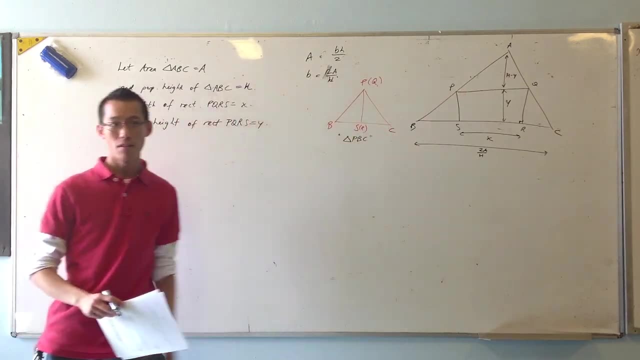 call this triangle PBC, And I can show that this triangle and the one at the top right, Can you see they're going to be similar, Right? You've got, because of this rectangle here, you've got parallel lines, right. 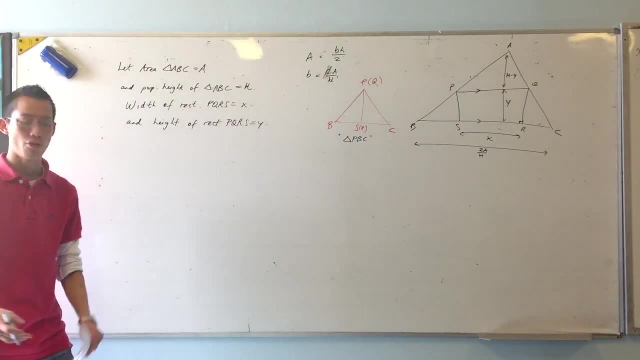 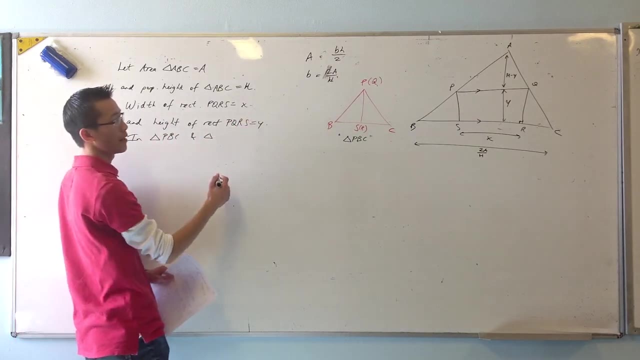 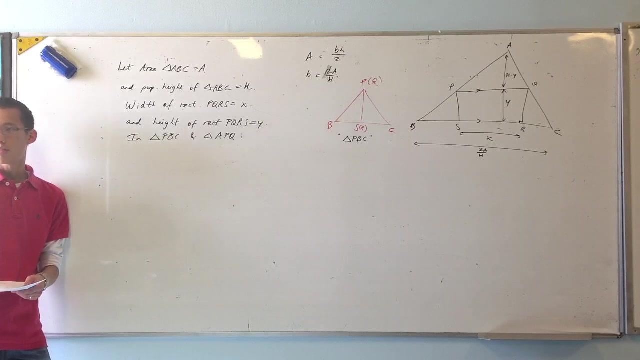 So you've got a whole bunch of corresponding angles which I'm going to show in a second. So let's have a look at this triangle: PN triangle, PBCN triangle, The one at the top, APQ. Okay, For similarity, all I need is two angles. 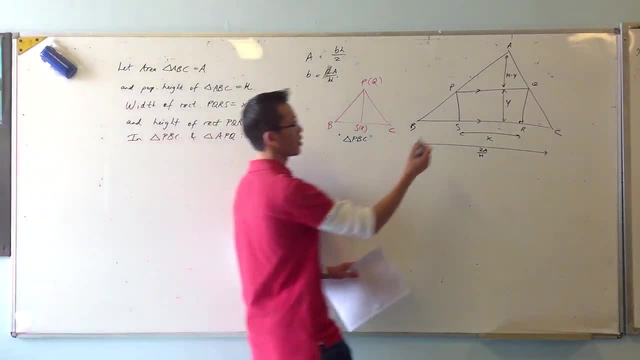 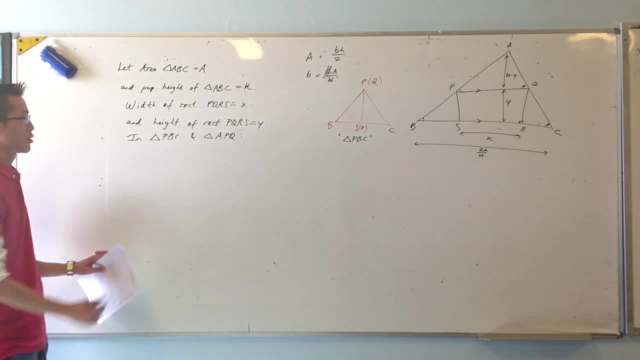 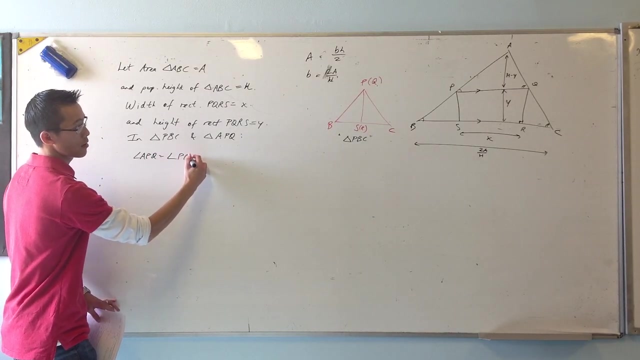 Right? So I'll just use corresponding angles to go this pair and this pair. Okay, You see that That's not too hard, Right? So let me just what would I actually write out. I'm going to say angle APQ is equal to angle PBC, because corresponding angles on those. 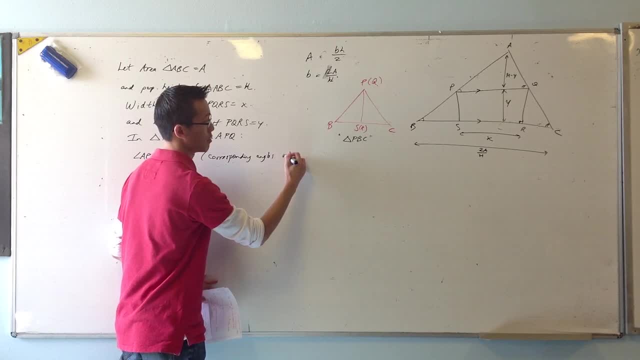 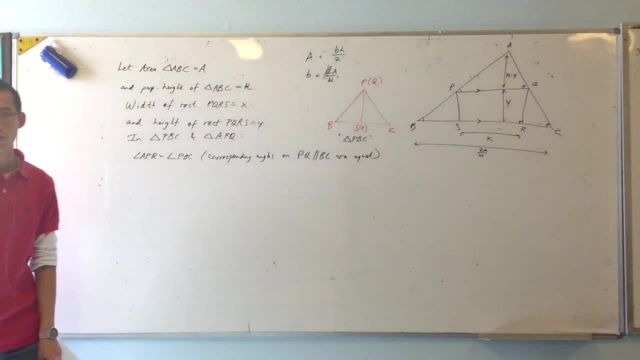 parallel lines, Right, Okay, So I'm going to say: angle PBC is equal to angle PBC is equal to angle R. Okay, I've been asked this a few times. Yeah, How come we aren't allowed to abbreviate abbreviations? 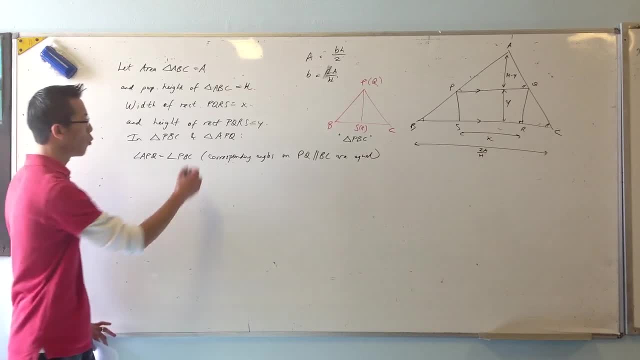 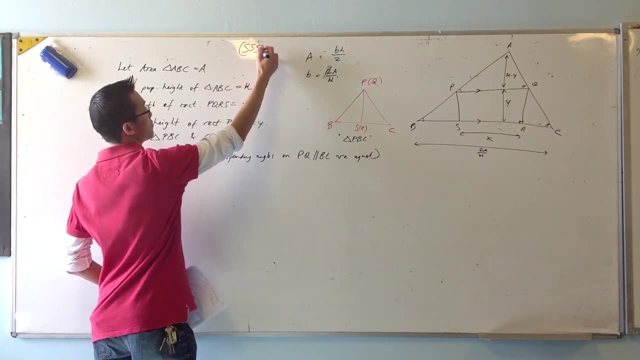 Abbreviations. I mean, we kind of do use abbreviations where there's no ambiguity, Right, But when there's like okay, for instance, if you saw this, okay, we allow that for congruence, but we don't allow it for similarity. 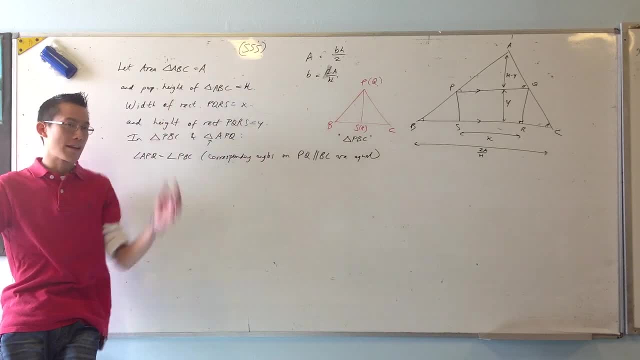 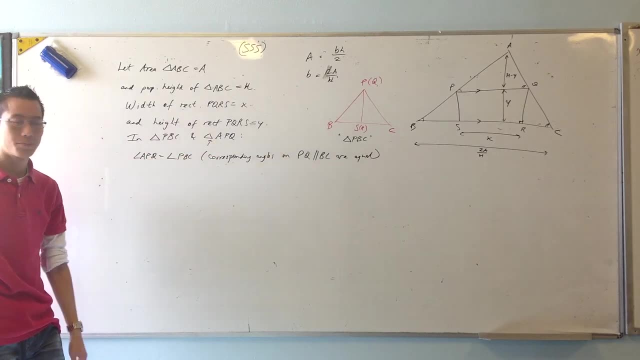 of similarity, because it's like side side, side. but what about them? The fact that they are in proportion. So when you abbreviate that, you lose some meaning. When you abbreviate this, you don't lose meaning, because it's like, yeah, OK. 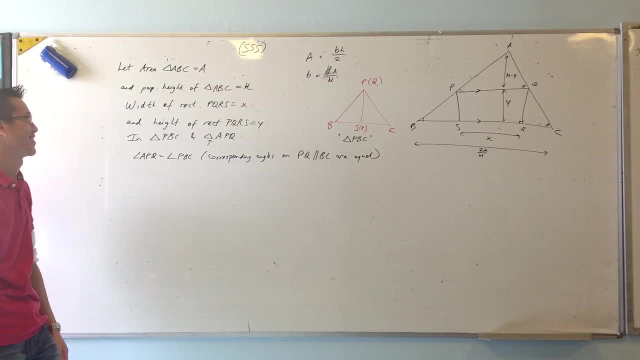 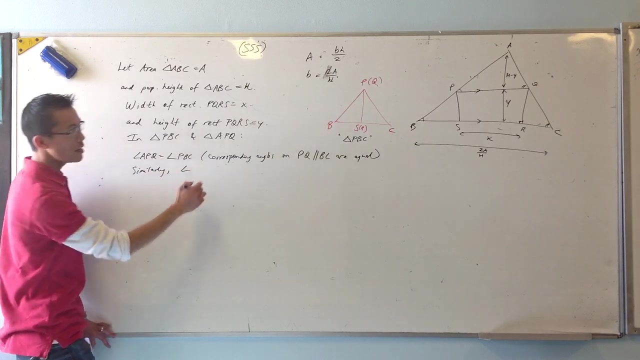 What's delta A? thank you, Thank you, OK With context. No, I'm not doing calculus. So therefore I've got those two angles equal. I can say similarly, because it's exactly the same reason, Angle A, Q, P, they're the opposite, ones are equal to angle PCP. 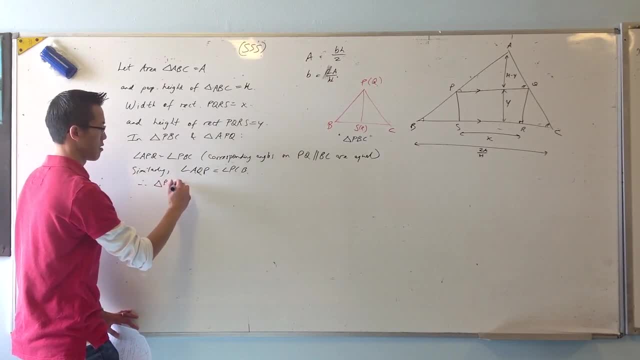 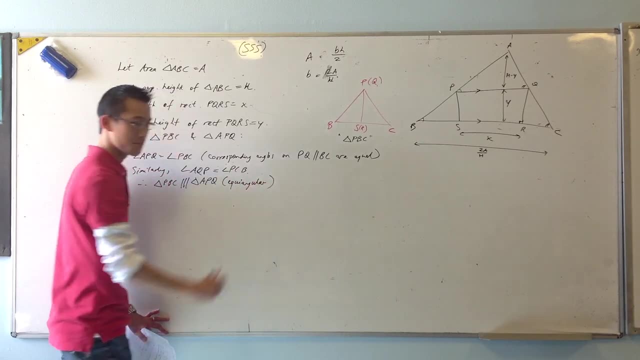 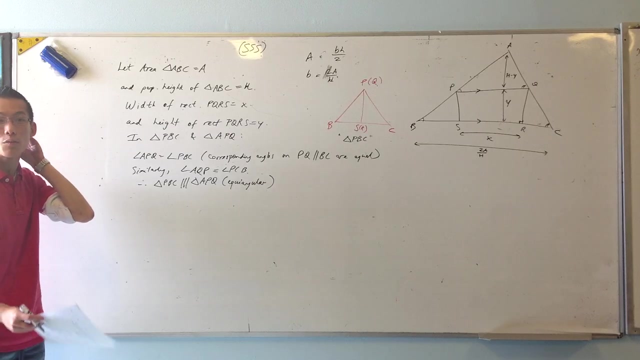 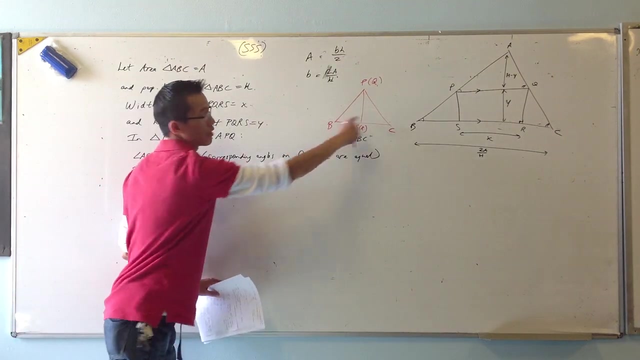 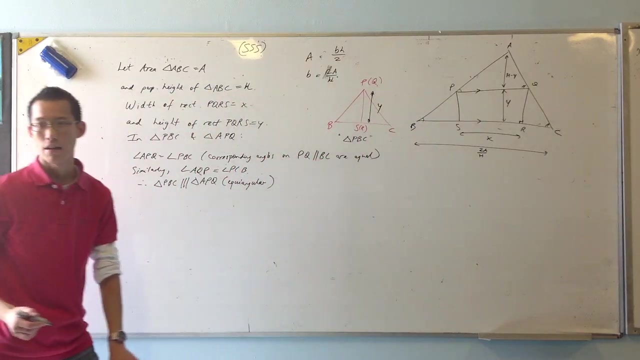 OK, So similar. OK So far, so good. Where am I going here? OK, When I've got these two similar triangles, I can relate a whole bunch of these variables and constants together. Namely This triangle here that I just introduced: its height is y. 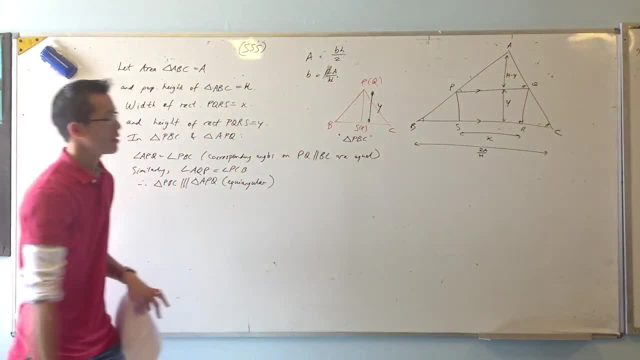 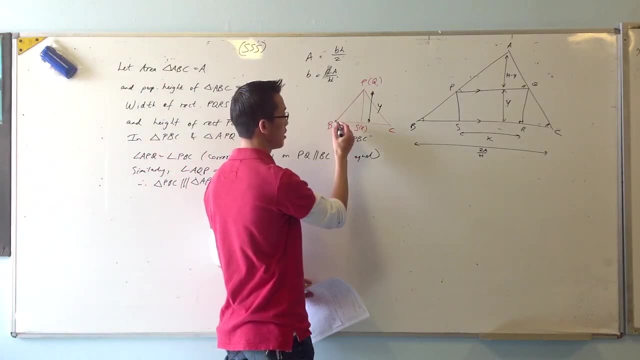 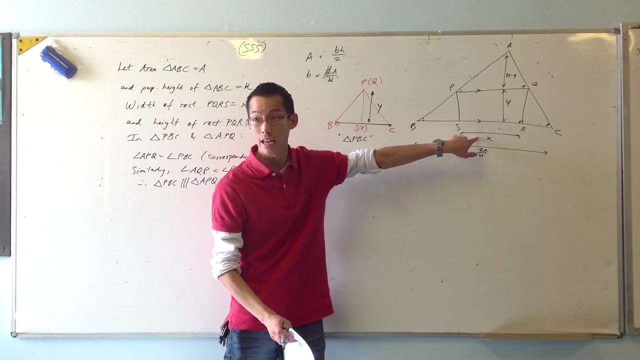 because I got it from here. Its base is the whole base of the whole triangle, minus the rectangle part which I cut out. So this base here, from here to here, that's the whole base and that's the rectangle part.